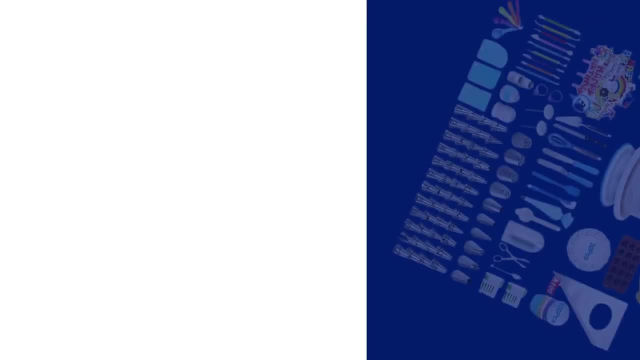 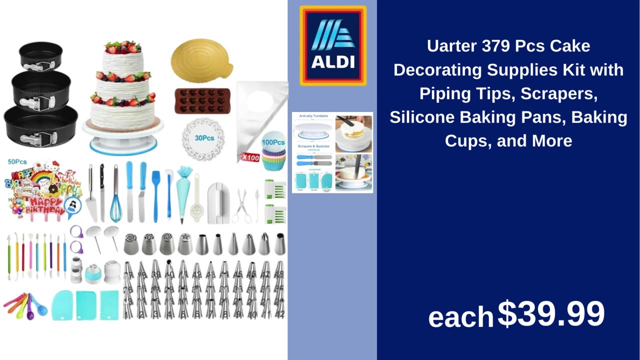 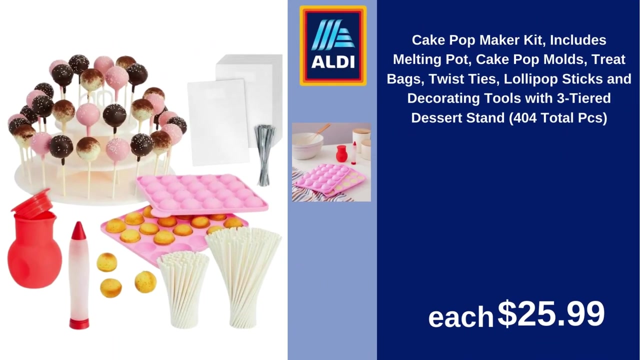 Puddings, Jellies and Chocolates- $90.99.. UARTER 379 PC's Cake Decorating Supplies Kit with Piping Tips, Scrapers, Silicone Baking Pans, Baking Cups and more- $39.99.. Cake Pop Maker Kit includes Melting Pot, Cake Pop Molds, Treat Bags, Twist Ties, Lollipop Sticks. 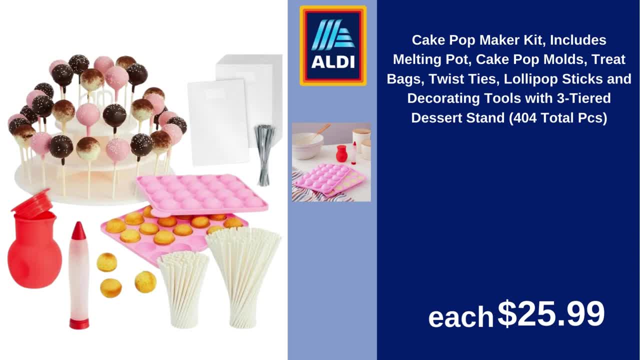 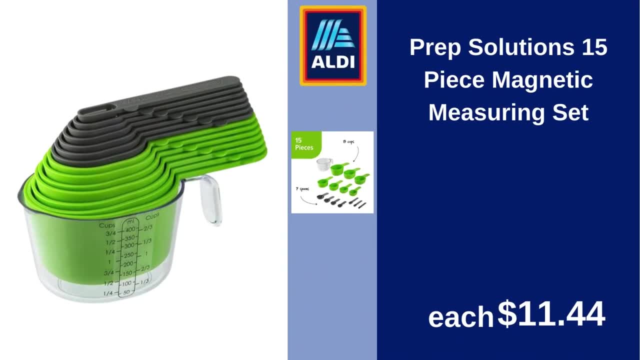 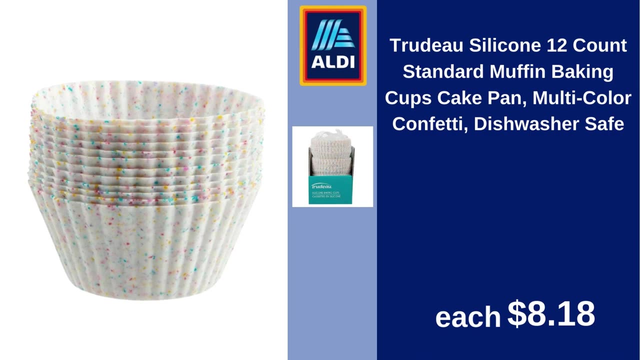 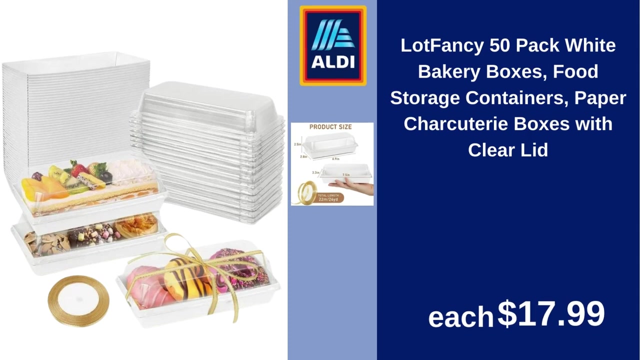 and Decorating Tools with 3-Tier Dessert Stand for 4 total PCs- $25.99.. Prep Solutions 15-Piece Magnetic Measuring Set- $11.44.. Trudeau Silicone 12 Count. Standard Muffin Baking Cups. Cake Pan, Multicolor Confetti- Dishwasher Safe- $8.18.. Lot Fancy: 50-Pack White Bakery Boxes- Food Storage. 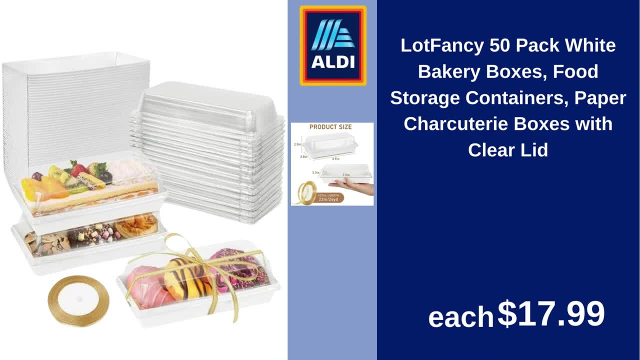 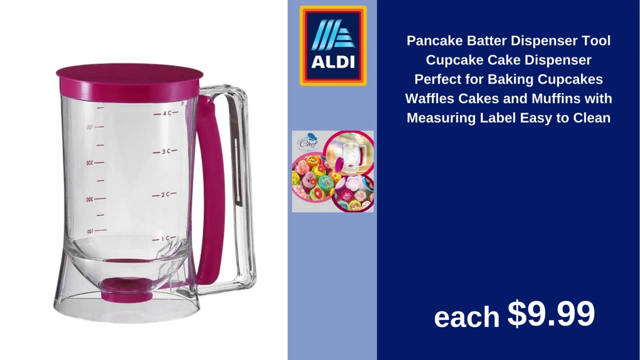 Containers. Paper Charcuterie Boxes with Clear Lid- $17.99.. Pancake Batter Dispenser Tool. Cupcake Cake Dispenser- Perfect for Baking Cupcakes, Waffles, Cakes and Muffins, with Measuring Label, Easy to Clean. 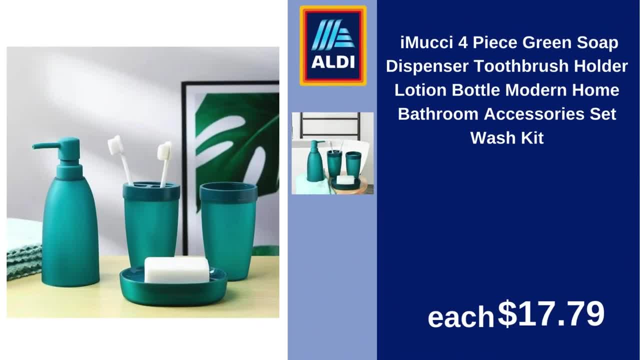 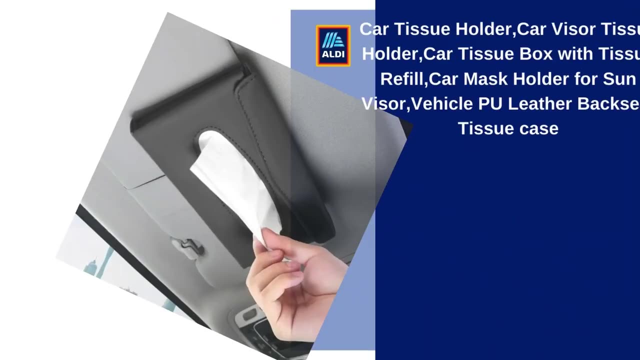 $9.99.. iMucci 4-Piece Green Soap Dispenser, Toothbrush Holder, Lotion Bottle- Modern Home Bathroom Accessories- Set Wash Kit- $17.79.. Car Tissue Holder- Car Visor Tissue Holder- Car. 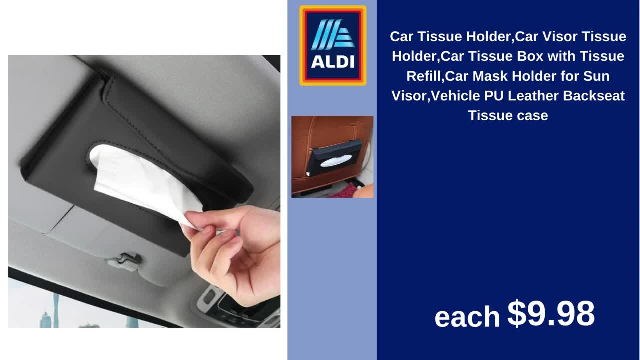 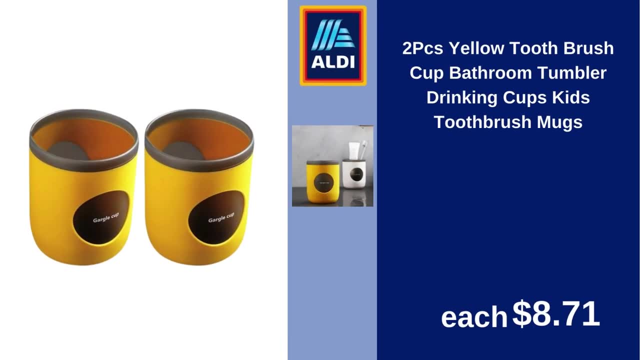 Tissue Box with Tissue Refill. Car Mask Holder for Sun Visor. Vehicle PU Leather Back Seat- Tissue Case- $9.98.. iMucci 4-Piece Yellow Toothbrush Cup, Bathroom Tumbler, Drinking Cups, Kids Toothbrush Mugs. 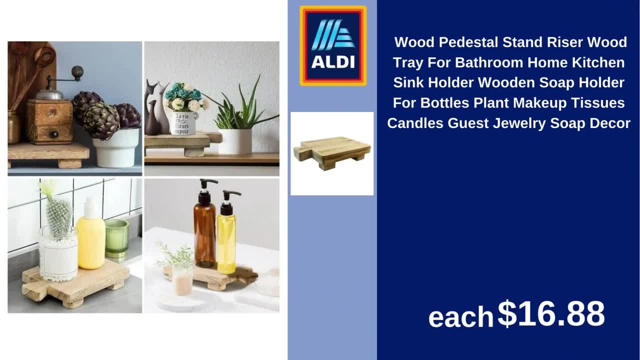 $8.71.. Wood Pedestal Stand Riser. Wood Tray for Bathroom, Home Kitchen Sink Holder. Wooden Soap Holder for Bottles, Plant Makeup Tissues, Candles, Guest Jewelry, Soap Decor. $16.88.. Ozomian Toilet Bowl Brush and Holder. Compact Toilet Cleaner Brush Set for Bathroom Deep. 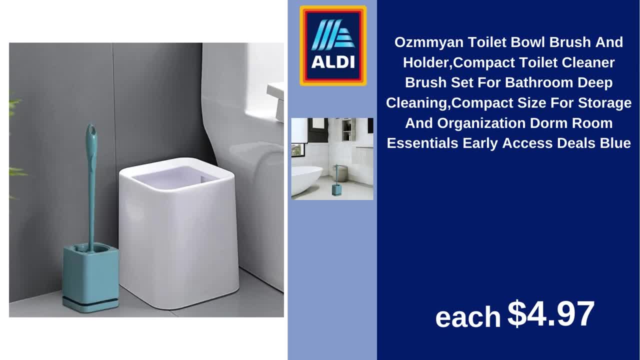 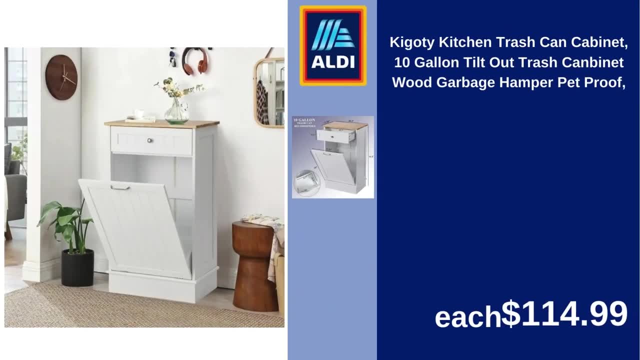 Cleaning, Compact Size for Storage and Organization. Dorm Room Essentials- Early Access Deals Blue- $4.97.. Kigoti Kitchen Trash Can- Cabinet Tessin Gallon Tilt-Out Trash Can- Binette Wood Garbage Hamper- Pet Proof- $114.99.. 5 PCs Kitchen Towel Holder: No Drilling Required, Self-Adhesive Round Towel. 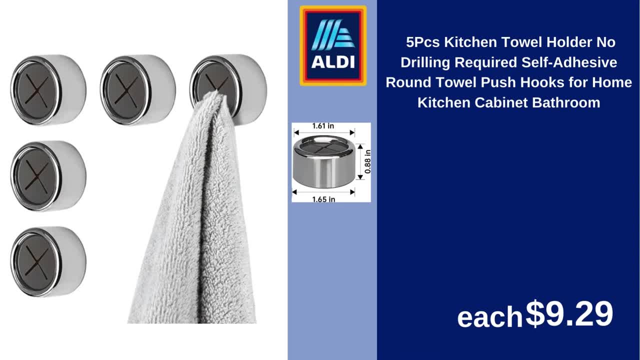 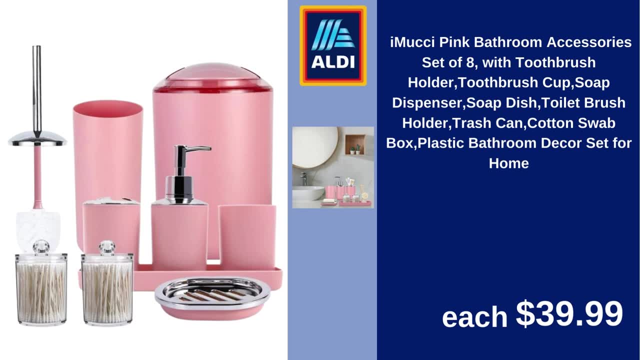 Push Hooks for Home: Kitchen Cabinet, Bathroom- $9.29.. iMucci Pink Bathroom Accessories- Set of 8 with Toothbrush Holder, Toothbrush Cup, Soap Dispenser, Soap Dish, Toilet Brush Holder, Trash Can, Cotton Swab Box, Plastic Bathroom Decor Set for Home- $39.99. Panda Kids 2 Piece Bath Towel. 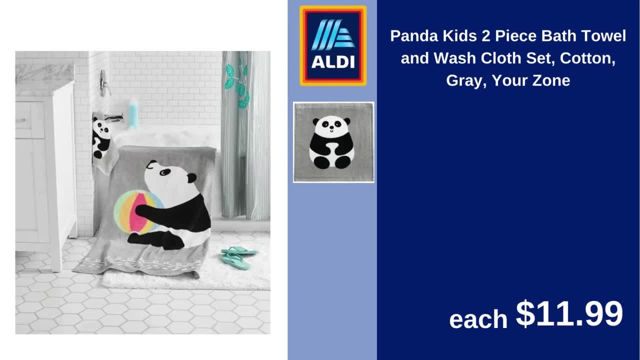 and Washcloth Set, Cotton Gray- Your Zone- $11.99.. By the way, 85% of our channel's viewers are not subscribed to our channel, and this makes us very sad. Don't forget to subscribe to the channel to support us and for more videos. 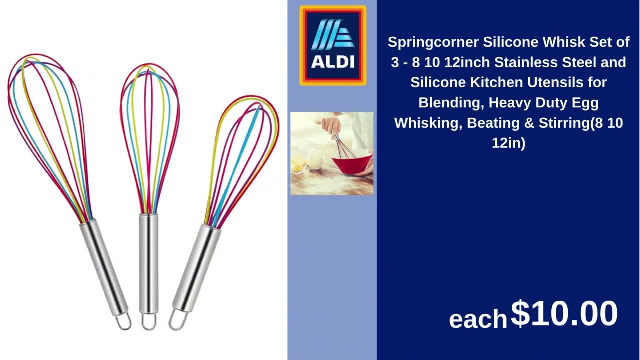 Spring Corner Silicone Whisk. Set of 3,, 8,, 10, 12-inch Stainless Steel and Silicone Kitchen Utensils for Blending, Heavy Duty Egg Whisking, Beating and Stirring- 8,, 10,, 12-in. $10.00. 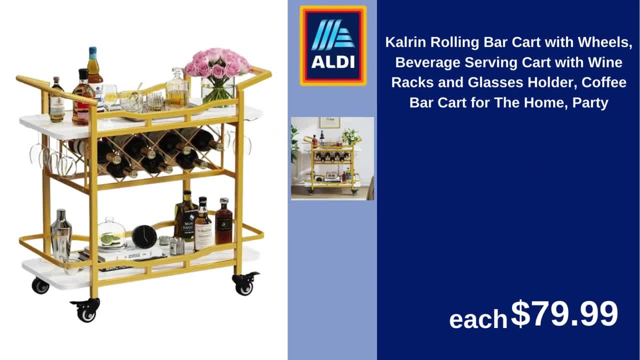 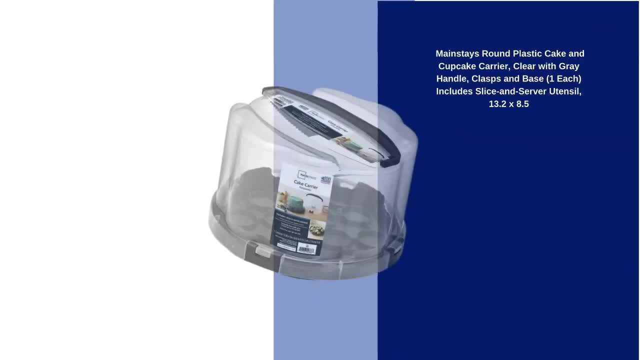 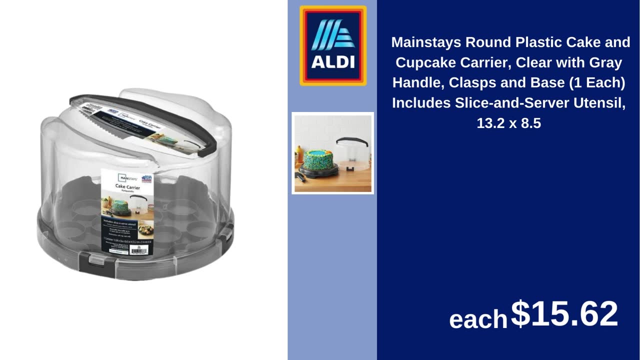 Calrin Rolling Bar Cart with Wheels. Beverage Serving Cart with Wine Racks and Glasses. Holder Coffee Bar Cart for the Home Party- $79.99.. Mainstays Round Plastic Cake and Cupcake Carrier with Gray Handle Clasps and Base one. each Includes Slice and Server Utensil: 13.2 x 8.5, $15.62.. 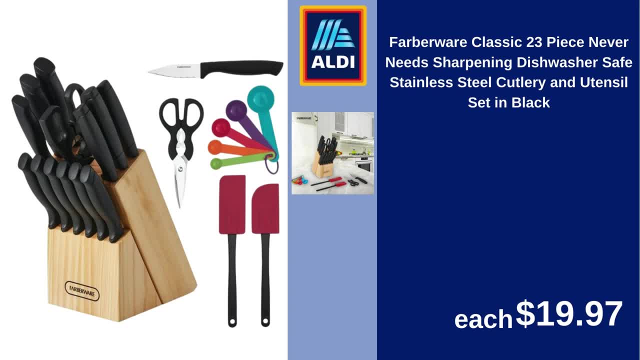 Farberware Classic, 23 Piece. Never Needs Sharpening Dishwasher Safe Stainless Steel Cutlery and Utensil Set in Black- $19.97.. Luxe Décor Kitchen Butcher Knife Stainless Steel, 7-inch. 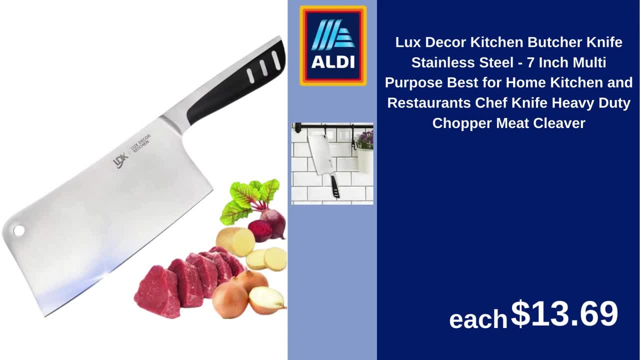 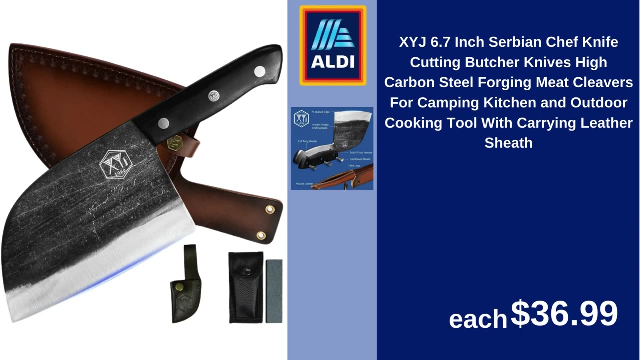 Multi-Purpose- Best for Home- Kitchen Chef Knife- Heavy Duty Chopper Meat Cleaver- $13.69,. XYJ. 6.7-inch Serbian Chef Knife- Cutting Butcher Knives- High Carbon Steel Forging Meat Cleavers for Camping, Kitchen and Outdoor. 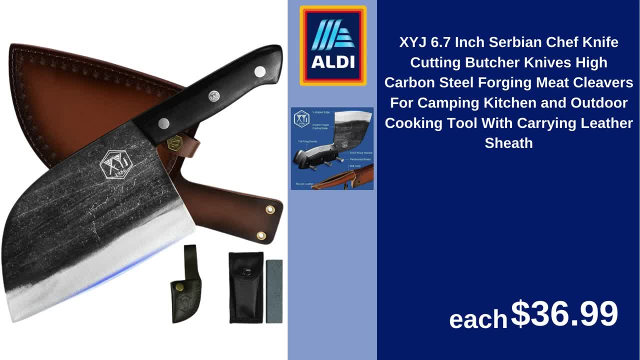 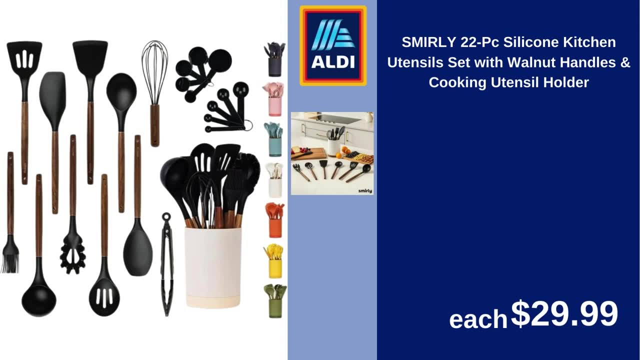 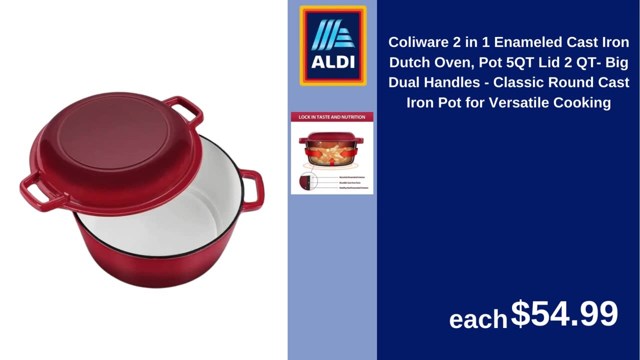 Cooking Tool with Carrying Leather Sheath: $36.99.. Smirely 22 PCC- $13.99.. Silicone Kitchen Utensil Set with Walnut Handles and Cooking Utensil Holder- $29.99. Colliware 2-in-1 Enameled Cast Iron Dutch Oven Pot 5QT, Lid 2QT. Big Dual Handles. 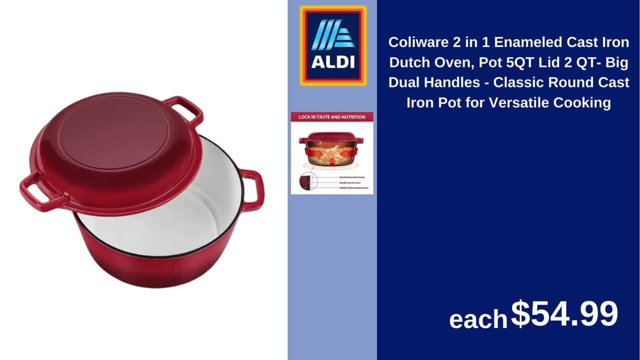 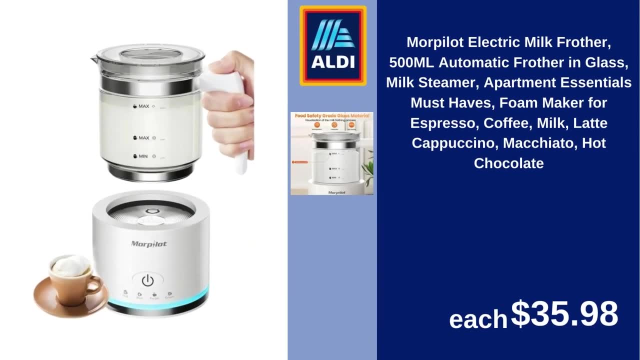 Classic Round Cast Iron Pot for Versatile Cooking- $54.99.. Morpilot Electric Milk Frother- 500ml. Automatic Frother in Glass. Milk Steamer. Apartment Essentials- Must-Haves. Foam Maker for Espresso, Coffee, Milk, Latte, Cappuccino, Macchiato, Hot Chocolate. 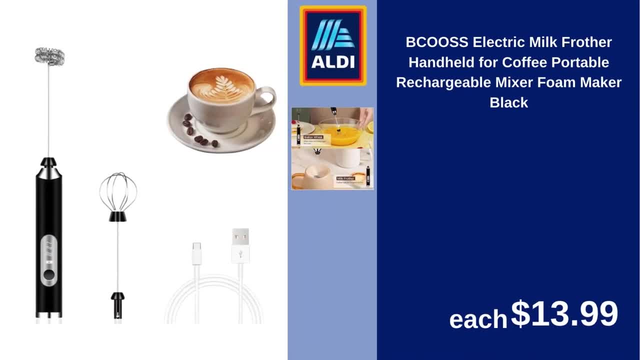 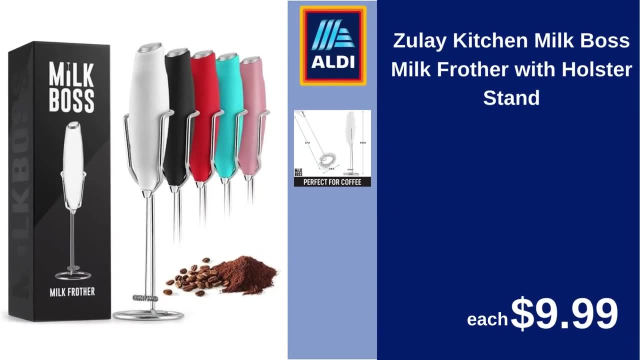 $35.98.. Beak Us Electric Milk Frother. Handheld for Coffee- Portable, Rechargeable Mixer. Foam Maker- Black- $13.99.. Zulay Kitchen Milk Boss Milk Frother with Holster Stand- $9.99. 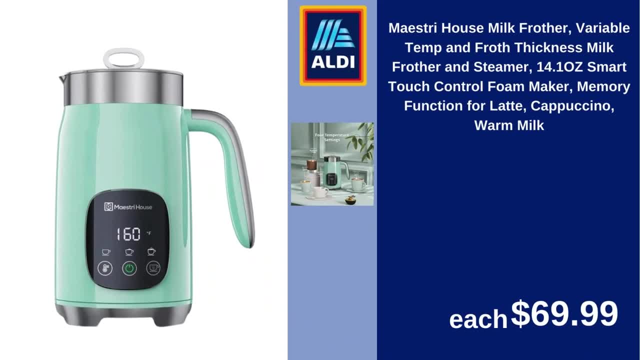 Maestri House Milk Frother- Variable Temp and Froth Thickness. Milk Frother and Steamer- 14.1-ounce Smart Touch Control Foam Maker Memory Function for Latte, Cappuccino, Warm Milk- $69.99. 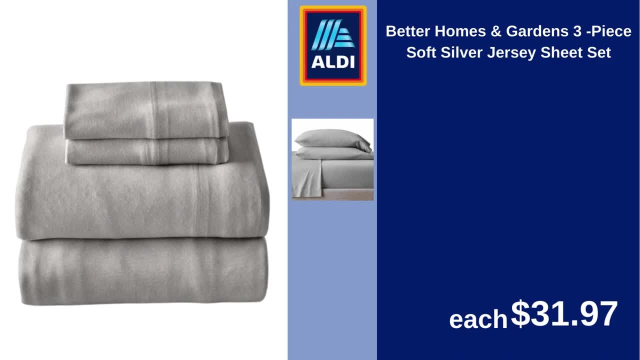 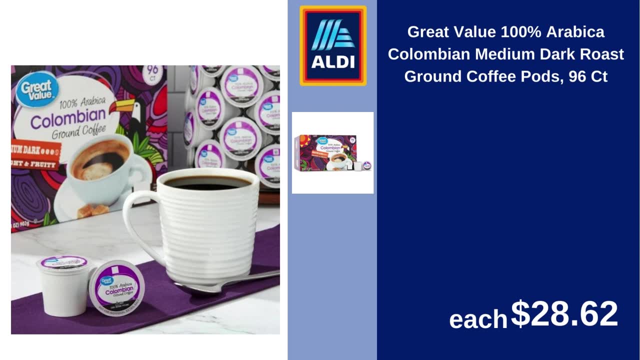 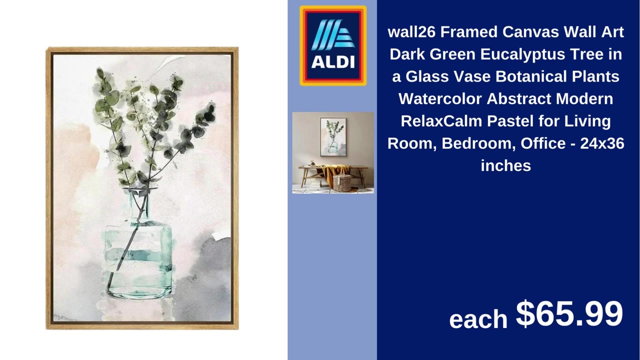 Better Homes and Gardens. 3-Piece Soft Silver Jersey Sheet Set: $31.97.. Great Value: 100% Arabica. Columbian Medium Dark Roast Ground Coffee Pods 96 count- $28.62.. Wall 26 Framed Canvas. Wall Art- Dark Green Eucalyptus Tree in a Glass Vase- Botanical Plants. 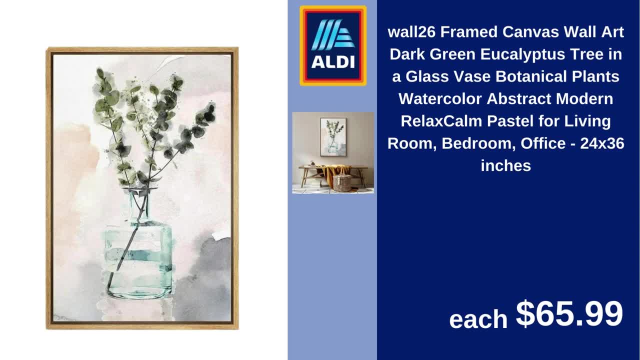 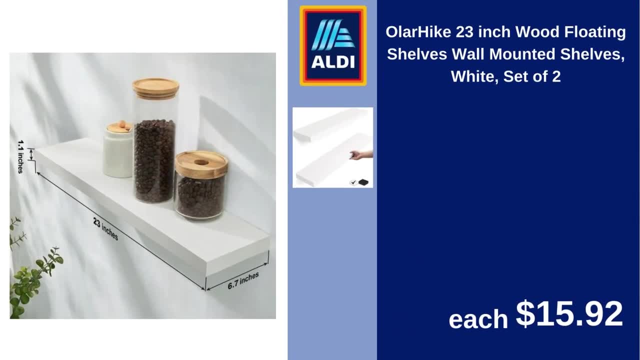 Watercolor Abstract: Modern Relax Calm Pastel for Living Room Bedroom Office- 24, 36 inches- $65.99.. Oler Hike- 23-inch Wood Floating Shelves, Wall-Mounted Shelves- White, Set of 2, $15.92.. 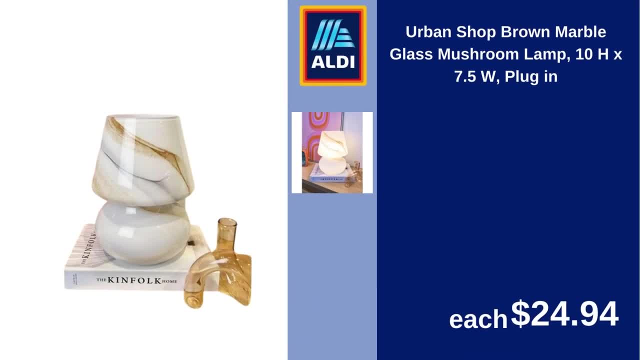 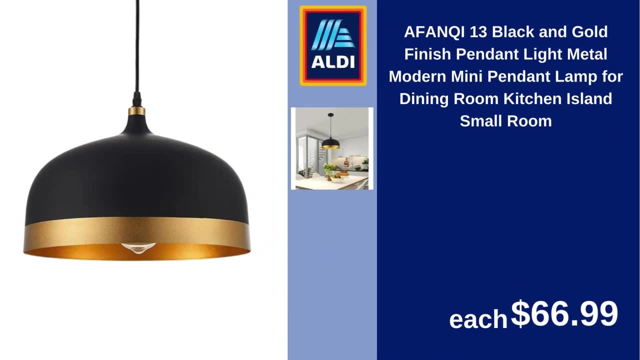 Urban Shop- Brown Marble Glass Mushroom Lamp 10HX. 7.5W. Plug-in- $24.94.. Afankee 13 Black and Gold Finish Pendant Light Metal Modern Mini Pendant Lamp for Dining Room, Kitchen Island, Small Room- $66.99.. 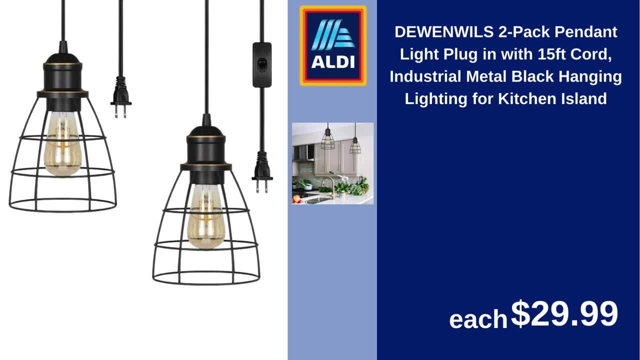 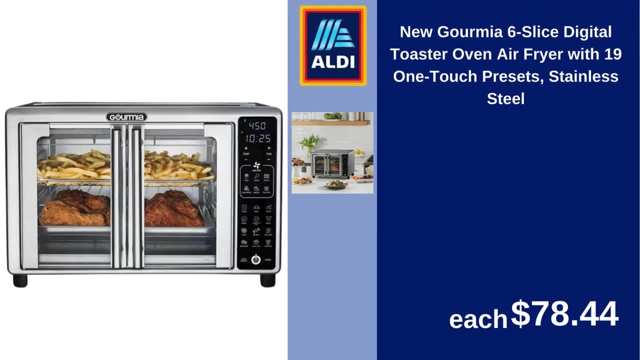 D1 Wills 2-Pack Pendant Light Plug-in with 15-ift Cord Industrial Metal Black Hanging Lighting for Kitchen Island- $29.99.. New Gourmia 6-Slice Digital Toaster. Oven Air Fryer with 19 One-Touch Presets- Stainless.